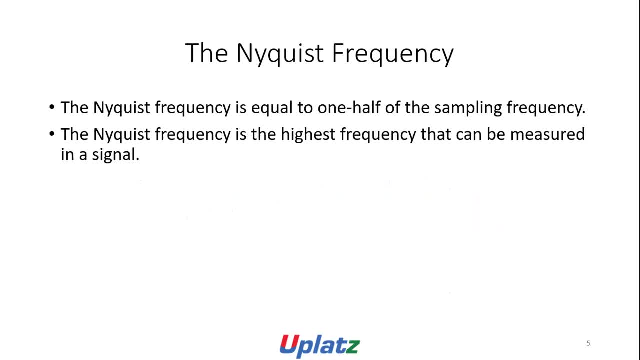 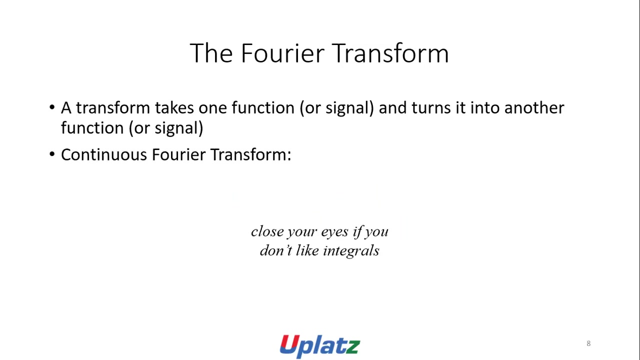 negative frequency. Negative frequency is equal to one half of the sampling frequency. Negative frequency is the highest frequency that can be measured in a signal. Periodic functions and signals may be expanded into a series of sine and cosine functions. A transform takes one function or signal and turns it into another function or signal. 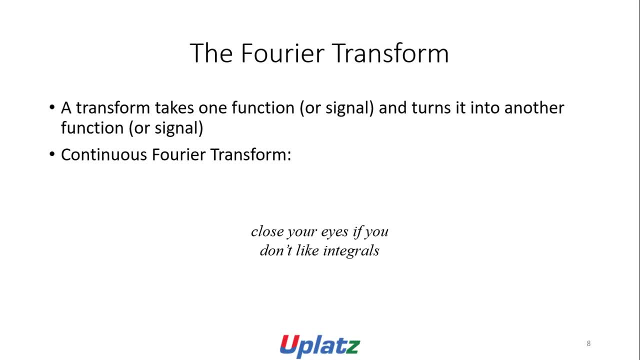 Continuous Fourier. transform closed airways, if you like integrals. h of f is equal to minus. infinity H of t is 2 pi t. Tribdf dt H of t is equal to minus. infinity H of t is equal to minus 2 pi I. trip dA. 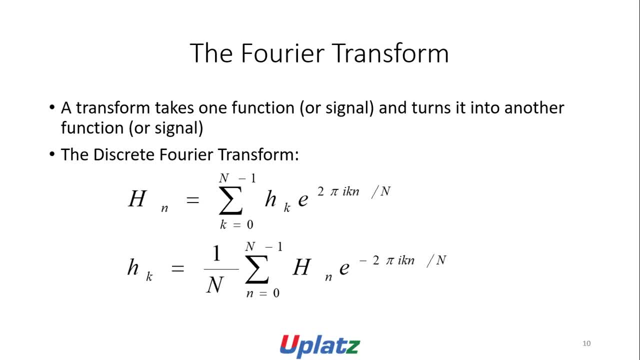 A transparent exponential function. h of n is equal to sigma. k is equal to zero to n minus 1.. k e power 2 pi i K n by n. where H k is equal to 1 by n. n, sigma n is 0 to n minus 1. h of n e to the power minus 2 pi e k n by n. 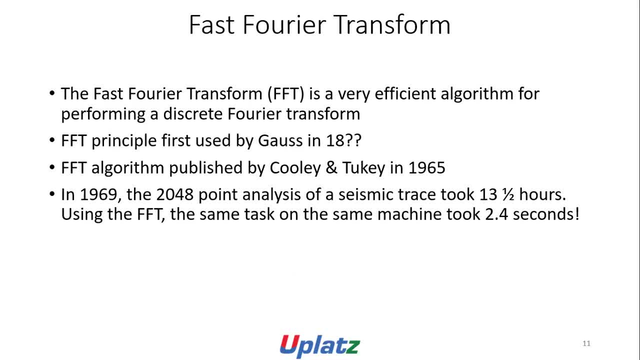 First Fourier transform. First Fourier transform is a very efficient algorithm for performing a discrete Fourier transform, FFT principle, first used by Koss in 18th century FFT algorithm published by Cooley and Tukey in 1965.. In 1969, the 24-point, 2048-point analysis of a seismic 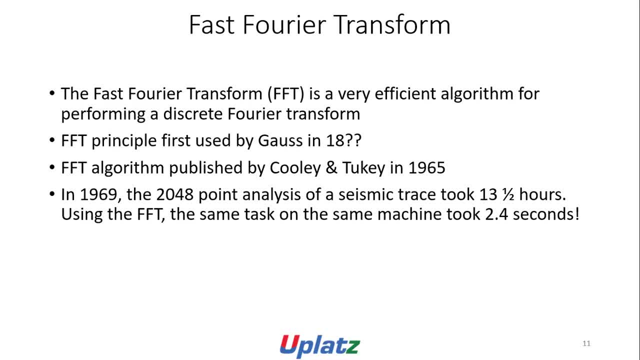 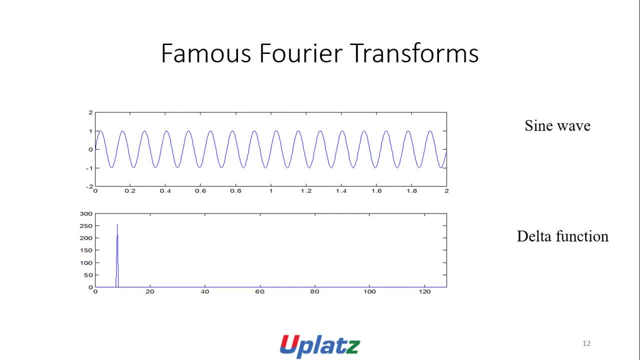 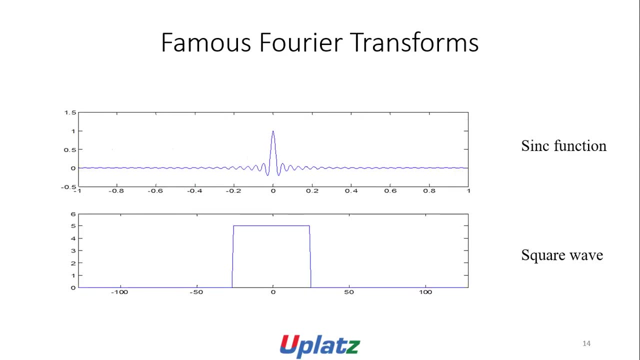 test took 13 and a half hours Using the FFT. the same task on the same machine took 2.4 seconds. Famous Fourier transform, sine wave and delta function is shown here. Gaussian and Gaussian function is shown here. Sink function and square wave function shown here. 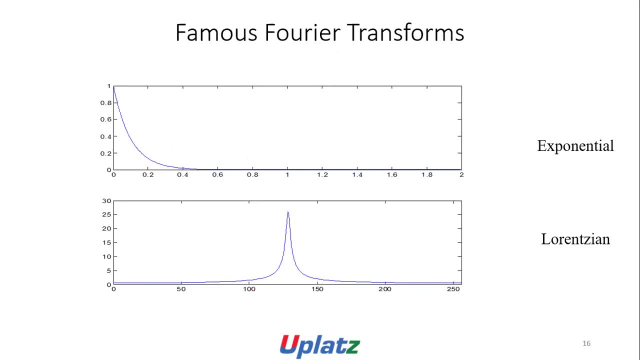 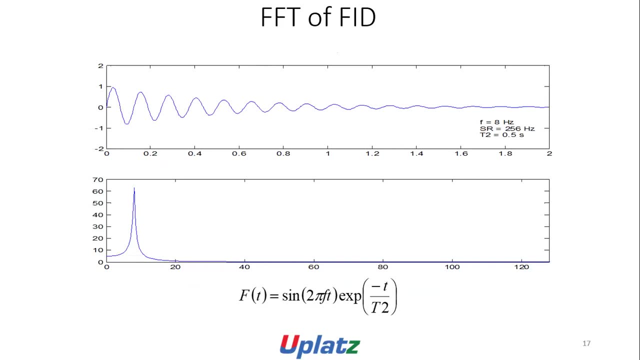 Sink function and square wave function shown here. Exponential and Lorentzian function is shown here. FFT of FID. FD is equal to sine 2, pi FD into exponential of minus 2 by T2.. F is equal to 8. 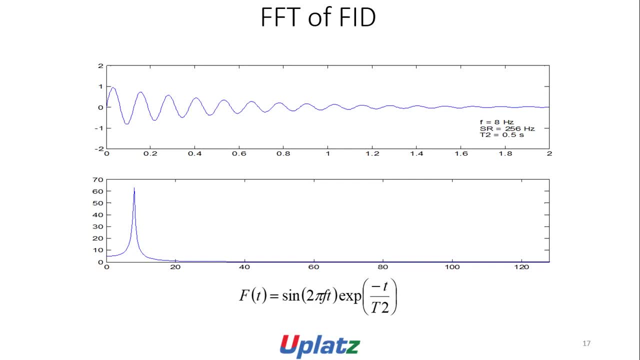 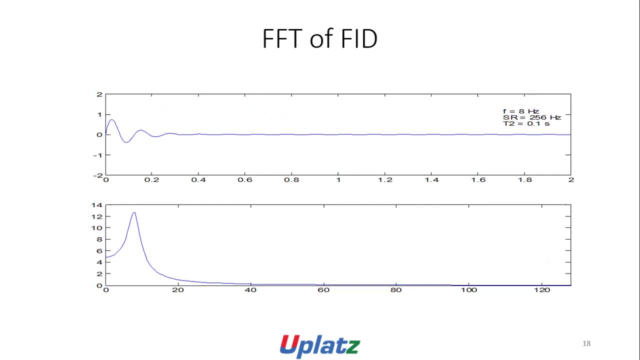 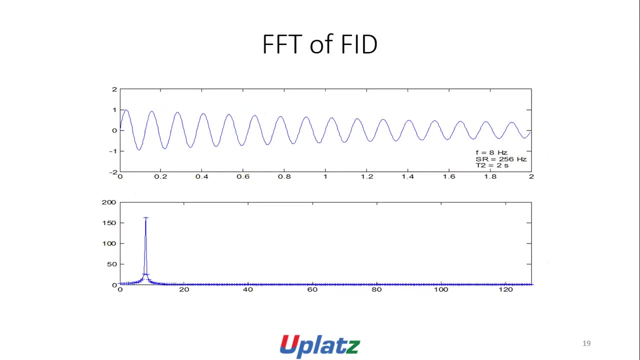 h. S is equal to 6 h. T2 is equal to 0.5 h and it is shown here So far. T2 is equal to 0.1 h. seconds is shown here Brownian figure And two seconds is shown here. Efforts are changing the sampling rate. 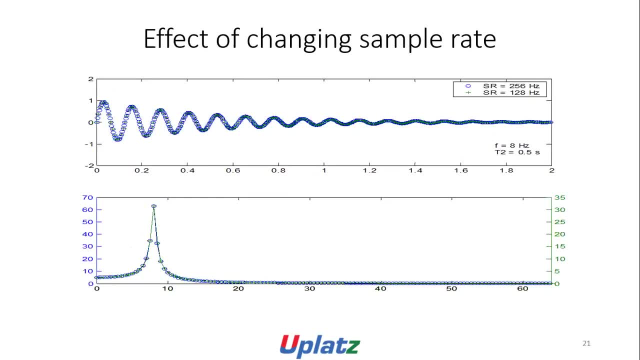 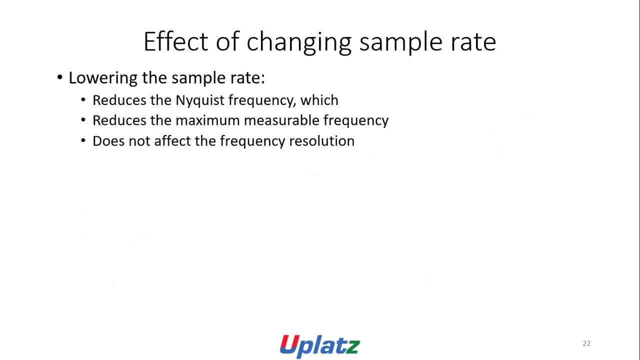 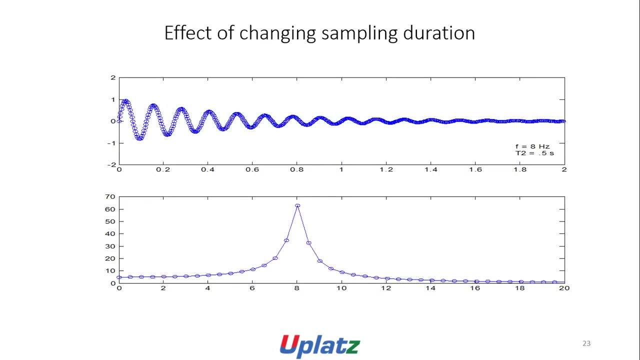 It is shown here. Another effect is shown here with the 128 hertz and 256 hertz. Lowering the sampling rate reduces the negative frequency, which reduces the maximum measurable frequency. It does not occur with the frequency of the solution. Effort is shown in the sampling. 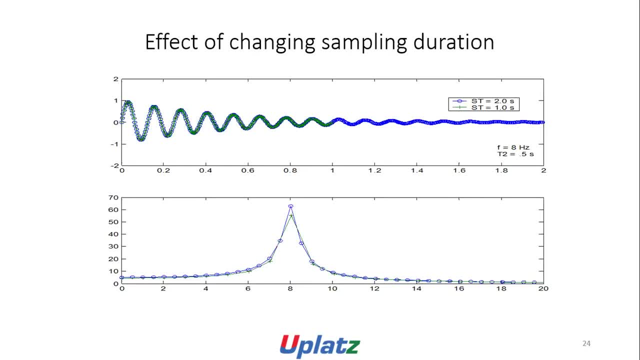 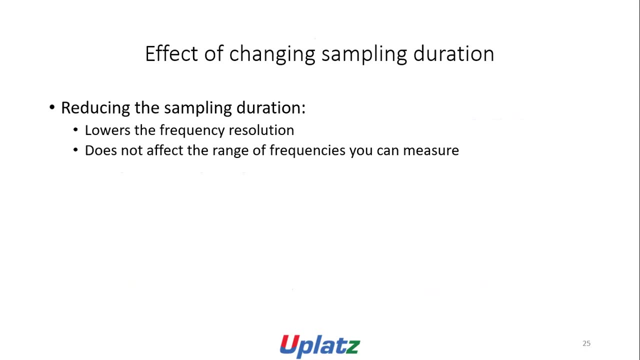 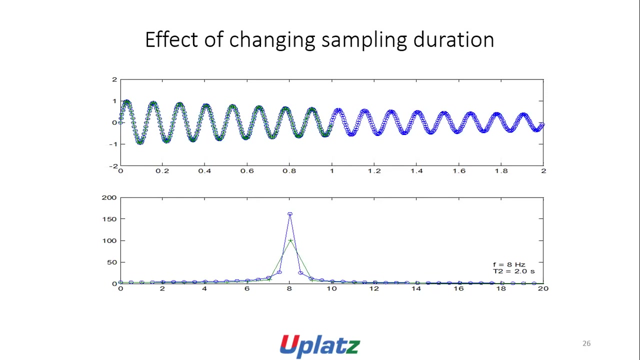 variation Providing the additional sample value in the test is shown here With: ST is equal to green value and ST is equal to two seconds and ST is equal to one second. Reducing the sampling duration- lower frequency in a solution- does not affect the range of frequency we measure. Then it is shown. the graphs are shown here: For sampling, two seconds and one second are shown here: 3 strain volume還有eras 2 Signalvolume per commission jumbo Boston and 0 mentre instrument response do not afect the range of the during measurement value of the same till淯級printing quickly increase levelsCheap Cond partido de boo SieHayt和 zure FADR in exibition is shown here. 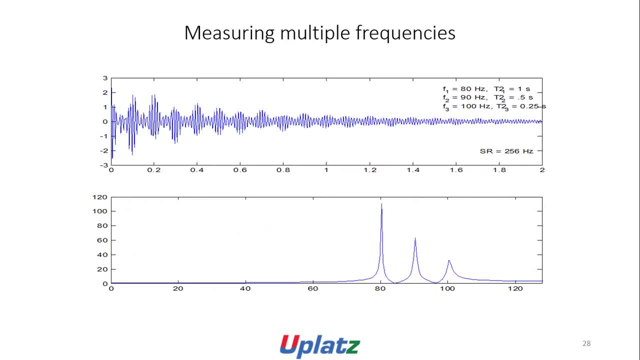 For f1 is equal to 80x. f2 is equal to 90x. f3 is equal to 100x. t2, 1 is equal to 1 second. t2, 2 is equal to 0.57,. t2, 3 is equal to 0.25 seconds, as shown here. Measuring of multiple. 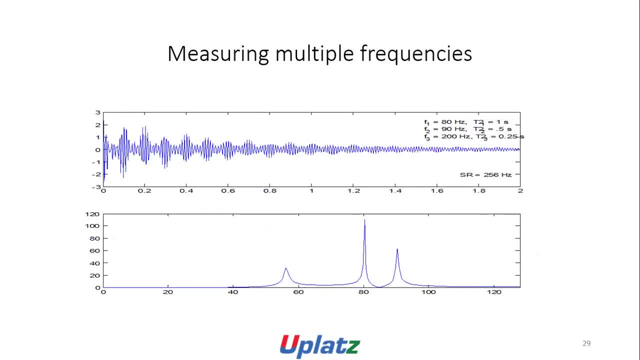 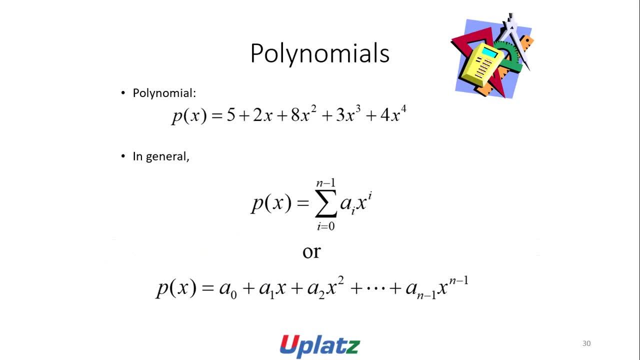 frequencies are possible. Here is another example. The sampling rate is equal to 6h. The polynomial p of x is equal to 5 plus 2x, 8x squared, 3x plus 4x, 4. in general, p of x is equal to. 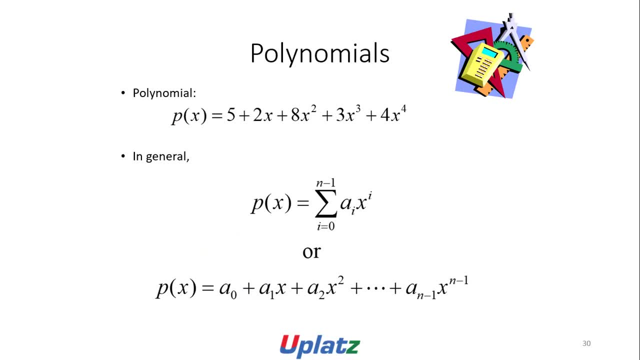 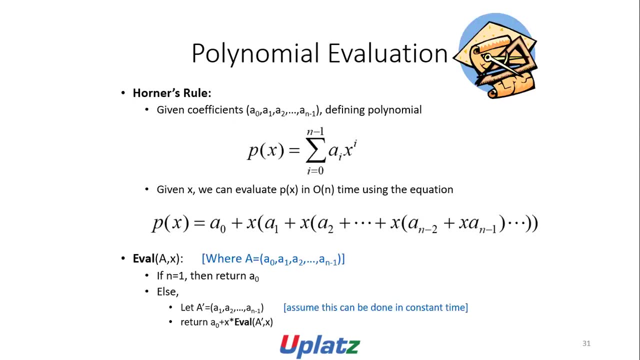 i is equal to 0 to n minus 1, a i, x, i, r, p of x is equal to a naught and a 1x plus a 2x squared plus a n minus 1 to x n n minus 1.. Polynomial aberration on a slope given a coefficient, a naught. 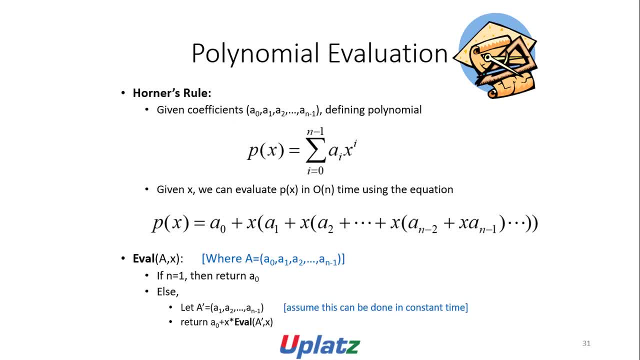 to a n minus 1.. Defining polynomial p of x i is equal to 0 to a n minus 1, a i x i Given x. we can evaluate p of x in order of n time Using the equation: p a naught x into a1 plus x into a2 plus x into a n minus 2 plus a x. a n minus. 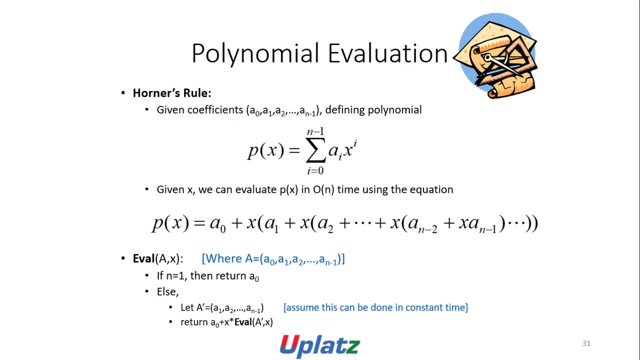 1, so on a by l a x, where a is equal to a naught, to a n minus 1.. If n is equal to 1, then return a naught, Else let a dash is equal to a1, a2, a n minus 1.. Return a naught is equal to x into. 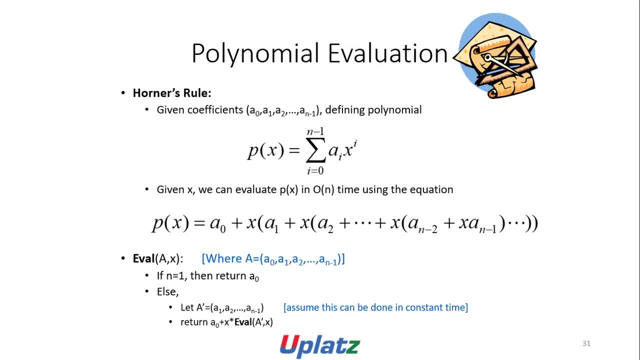 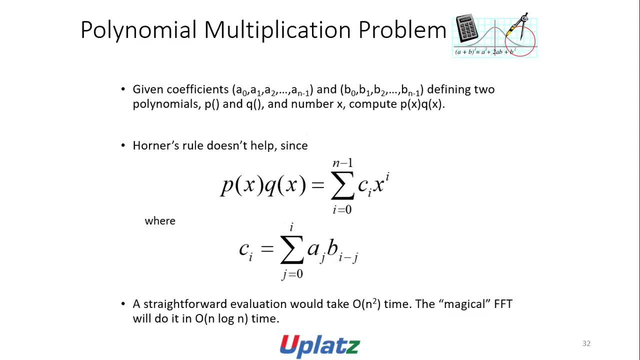 a, l, a dash, a transpose x. Assume this can be done in constant. Given the coefficients a naught to a n minus 1, p a naught b a n minus 1,, depending on the two polynomials p a and q and number x, compute p of x, q of x. 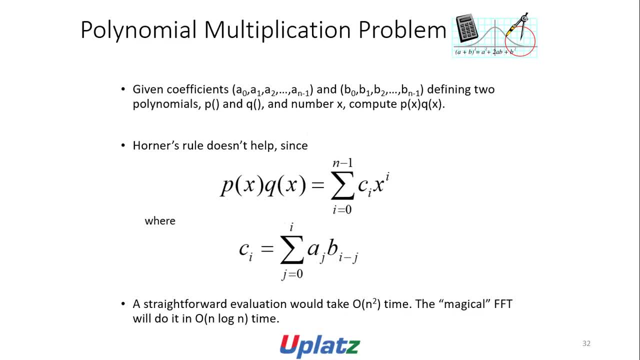 Arnold's rule does not help. since p of x is equal to a, i is equal to 0 to n, a n minus 1 c a, x i, where c? a is equal to g, is equal to 0 to n i. a of a, j into p a minus j A straighter. 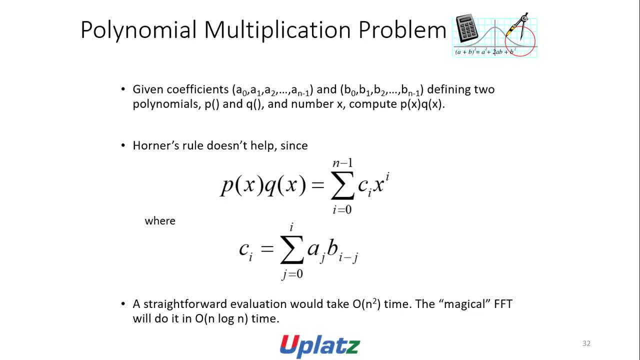 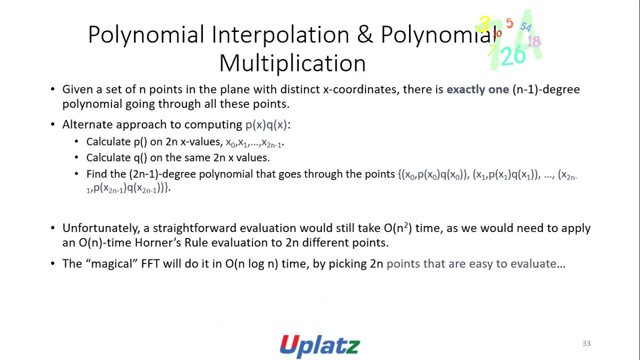 derivative will take the order of n. squared. The magic, the magical f of p will do it in order of n. log n time, Polynomial interpolation and polynomial multiplication. Given a set of n points in the plane with distinct x coordinates, there is exactly one n minus 1 degree polynomial going. 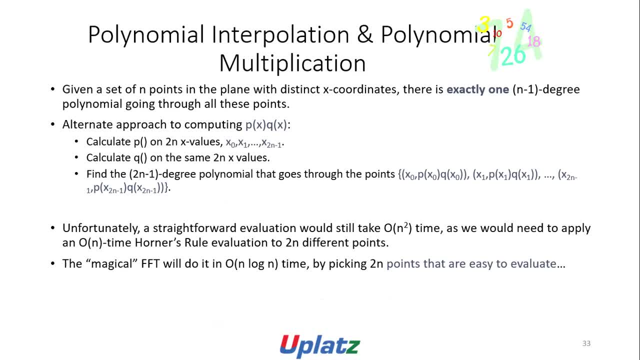 through all this point. Alternate approach to computing p of x, q of x is: calculate p on two n x values and calculate p on the same two n values. Find two n minus 1 polynomial and thus through the points x, p, naught, p x, naught, q, naught, x, naught, p x, 1 x, 1, p x, 1, p x, 1 x, 1.. 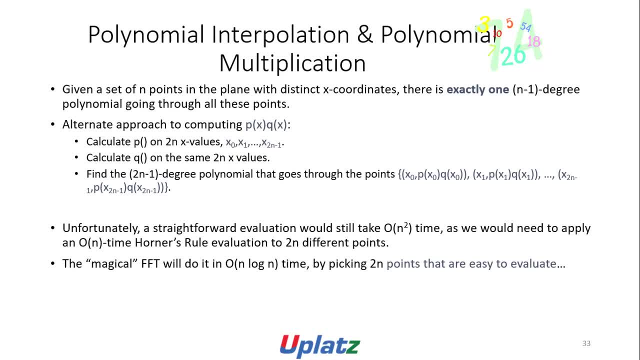 Unfortunately, a straighter derivative will still take the order of n squared time, as we would need to apply an order of n time- Arnold's rule evaluation- to two n different points. The magical f of p will do it in order of n log n time by picking two n points that are easy to evaluate. 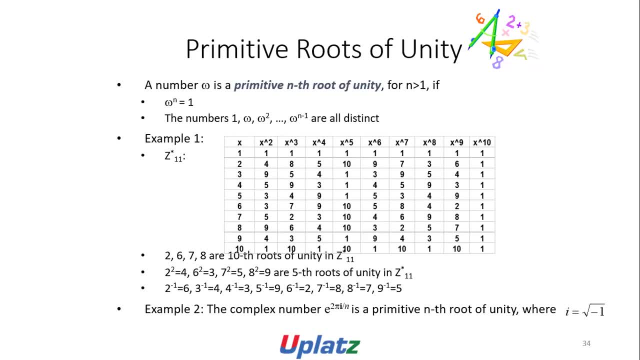 A number omega is permitting n through the community part, and this then one f omega power n is one. the numbers one are all distinct. is that one? one star is shown here: two, six, seven, eight, ten groups of unity in zero: one. two square is four, six square is one. 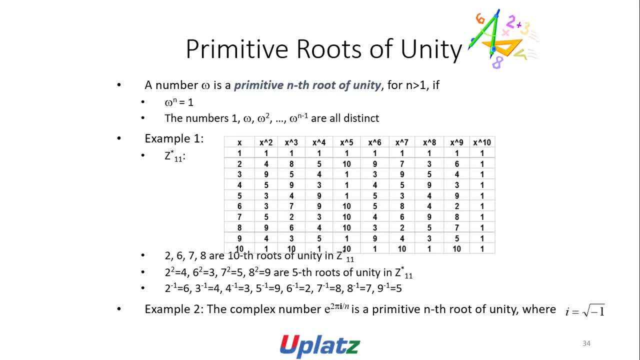 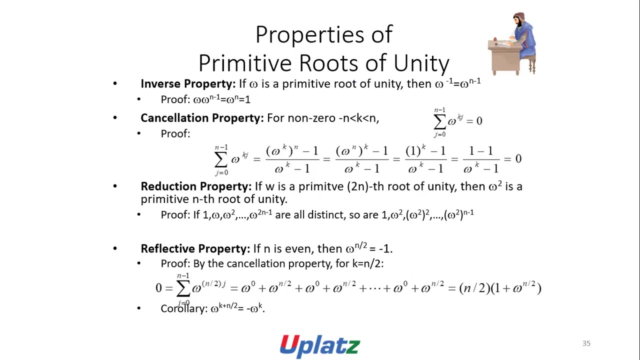 three and so on. example: the complex e power two a by n is primitive n through w, where i is one square root of minus one. What is the probability program of cellular technology? 하나 um Translation property For non-zero of k Haniabhi malpani. 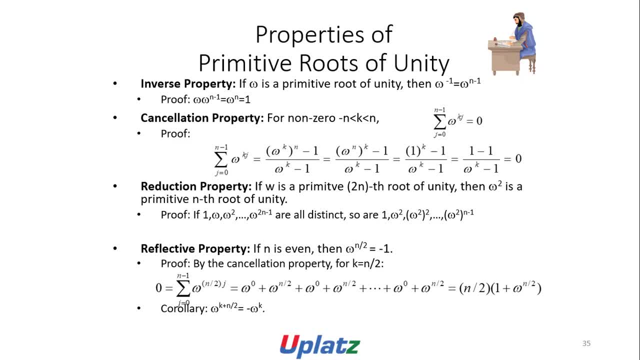 only less than n. sigma j is the zero to n minus one. half omega kj is equal to zero. same space. sigma h. sigma j is equal to zero to k. omega kj n minus one is equal to omega k power n minus one by omega k minus one. omega k power n. omega power n. power k minus one by omega k minus. 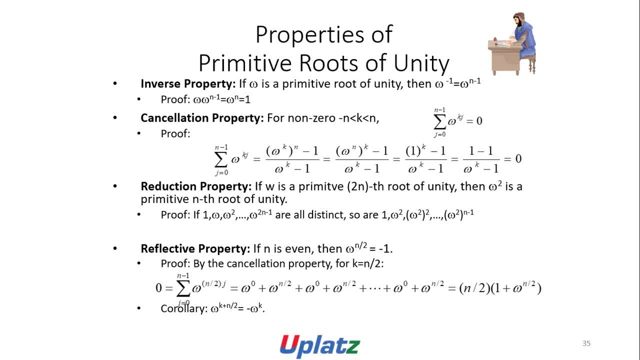 one is equal to one power. k minus one by k minus one is equal to one. minus one. by omega, k minus one is equal to zero. If w is primitive to the nth root of unity, then omega square is a primitive nth root of unity. So if one omega n square, or this and omega square, 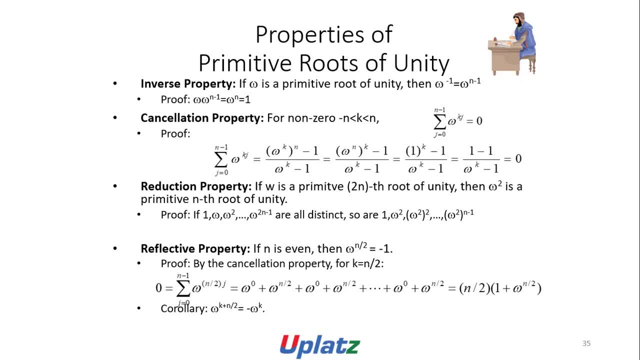 minus n, minus one, so r one omega square, omega square, so on. If n is even, then omega, n by two is equal to minus one. By cancellation, property for k is equal to n by two. we get the corollary omega k power. 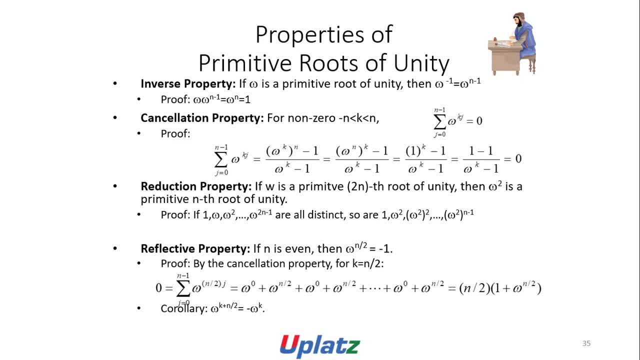 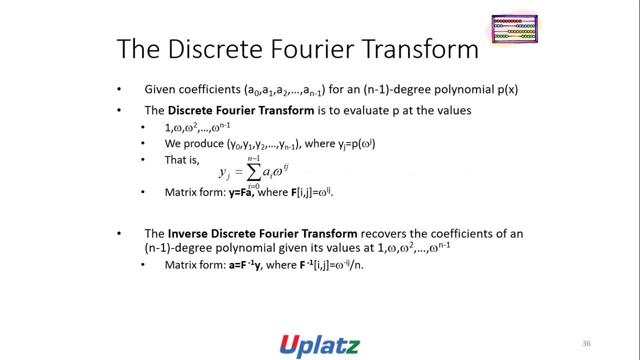 Okay, Okay, plus n by 2 is equal to omega minus omega power k. The discrete Fourier transform, given coefficients a naught to a n minus 1 power n, n minus 1, they get a polynomial to m. The discrete Fourier transform is to get the p values at omega 1, omega, omega, square omega. 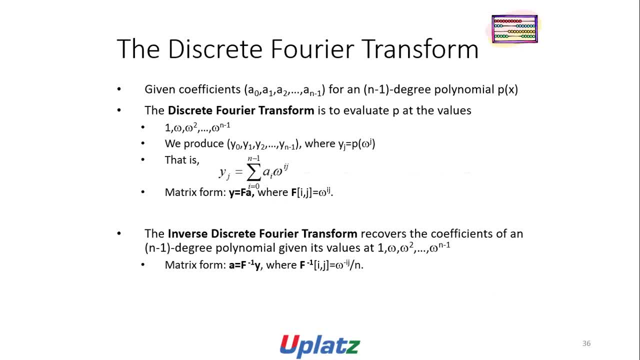 n minus 1.. We produce y naught to y, n minus 1, where y is equal to p, omega power, j, That is where j is equal to sigma, t is equal to 0 to i is equal to 0 to n minus 1. a i, omega. 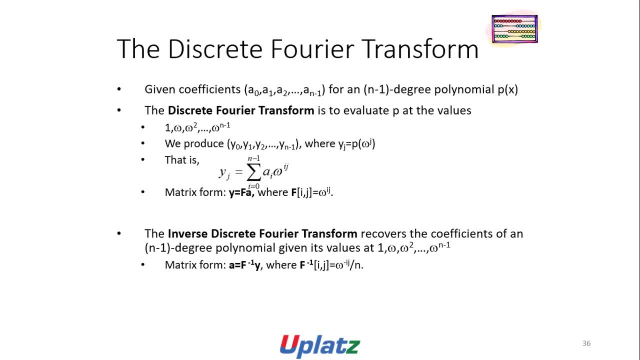 i- j. Matrix form: v is equal to f. i of j is equal to omega i- j. The inverse discrete Fourier transform requires: the coefficients of: n: Inverse is equal to 1, given its value at 1 omega omega square omega n minus 1.. Matrix a: f inverse y, where f inverse is i, j is equal. 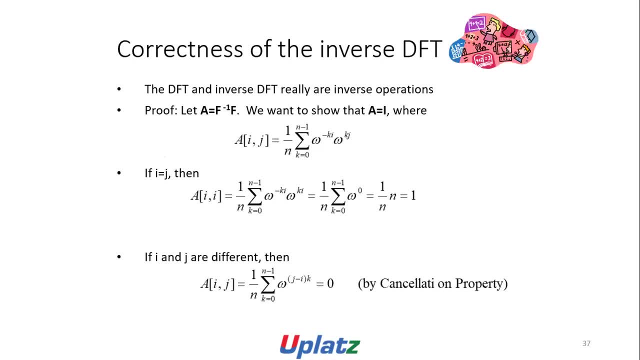 to omega minus i, j by n. Correctness on inverse DFT. the inverse DFT and inverse DFT are inverse operations. That is what we have in this draft. We want to show that a is equal to i, where a, i, j is equal. 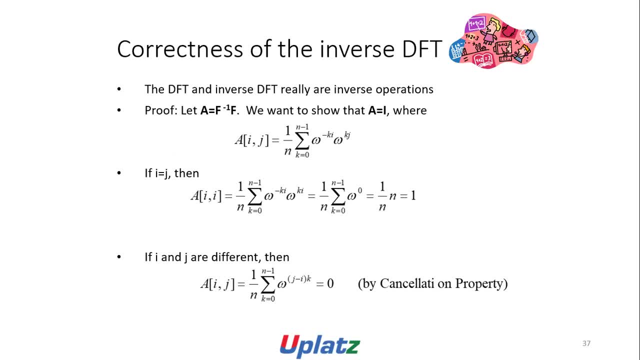 to 1 by n. k is equal to 0 to n minus 1. omega minus k. i. b into omega k j. If i is equal to j, then a i is equal to 1 by n. k is equal to 0 to n minus omega minus k. i into omega. 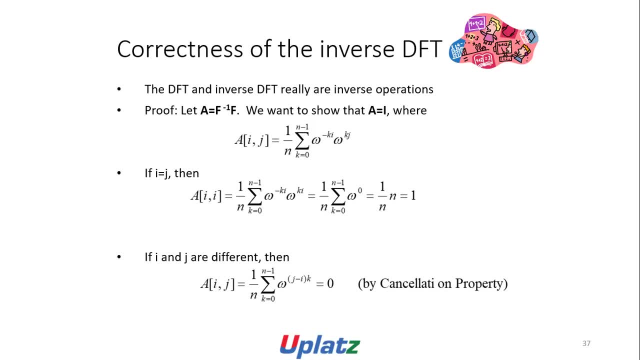 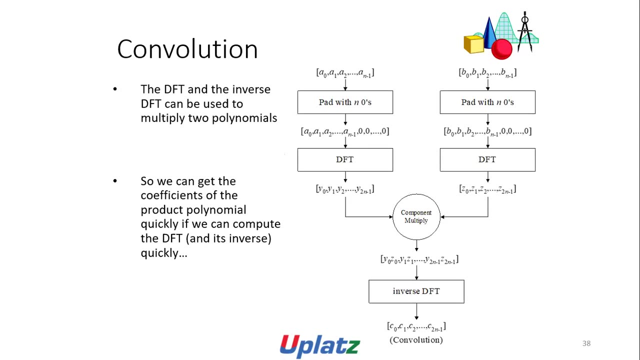 k i is equal to 1 by n. k is equal to 0, to omega n minus 1 over omega 0 is 1 by n by n is 1.. If a and g are different, then it will be equal to 0. by cancellation property Analyzing the DFT and inverse DFT can be used to multiply. 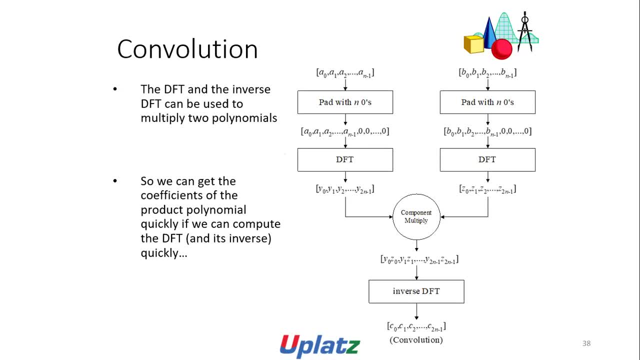 two polymers so we can get the quotient of the product polymer quickly. if we can compute the DFT and inverse DFT quickly, a naught, a n minus 1 b naught, n minus 1, paired with n zeros. paired with n zeros, it becomes a n i a n i. a naught to a n minus 1 0, 0, 0 b naught. 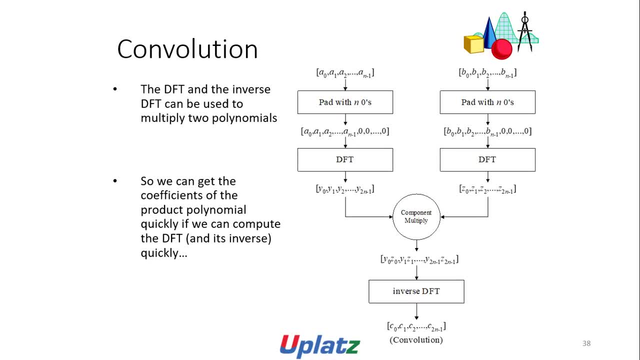 dft, dft. then we get y naught to y to n minus 1 is a naught, is a 2 minus 1 component multiplying then y naught is a, naught, y 1. inverse DFT, c naught, c, 1, c, 2 convolution. 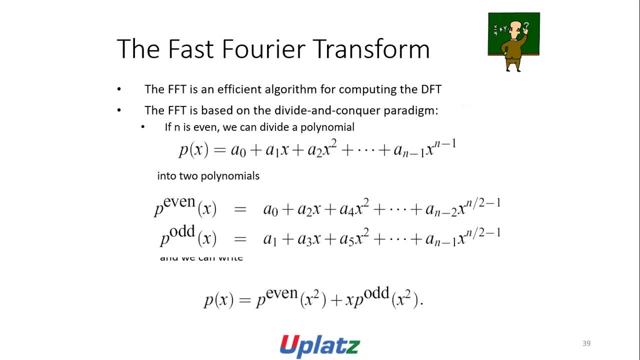 Fast Fourier transform. the FFT, is an efficient algorithm for computing the DFT. The FFT is based on the Debye-Conkoperadion. If n is even, we can divide. the polynomial p of x is equal to a naught a 1 x a 2 x. squared a n minus 1 as p e 1 is equal to a naught e 2. 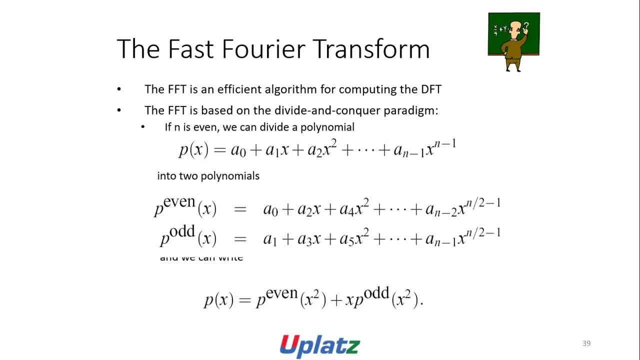 a 4 a n minus 2.. p out is equal to a 1 a 3 a 5 and so on. So p of x is equal to p e 1 into x squared, plus x into p out into x squared After. the FFT algorithm is shown here the: 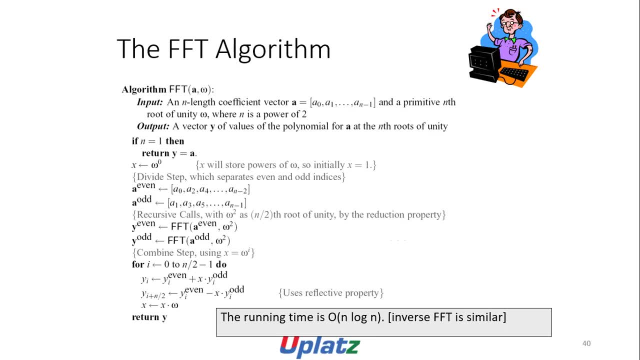 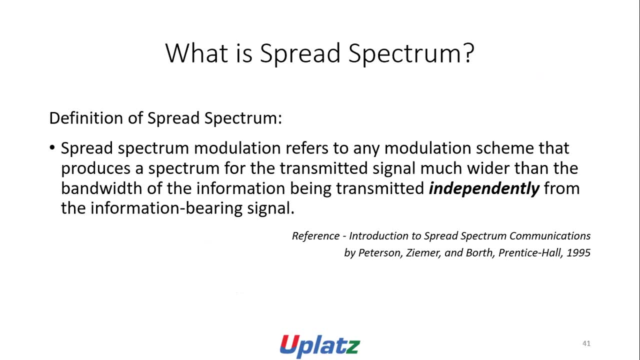 running time is 0.. This is the out of the out of n log n. You know FFT is similar. What is spectrochrome? Debye-Conkoperadion spectrochrome? Spectrochrome modulation requires to any modulation scheme that produces a spectrum for transmitter signal much wider than the bandwidth of the information. 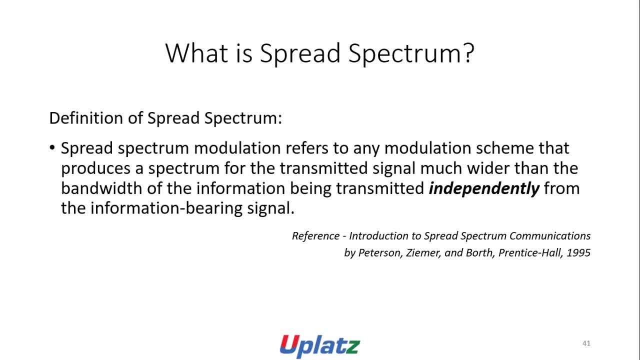 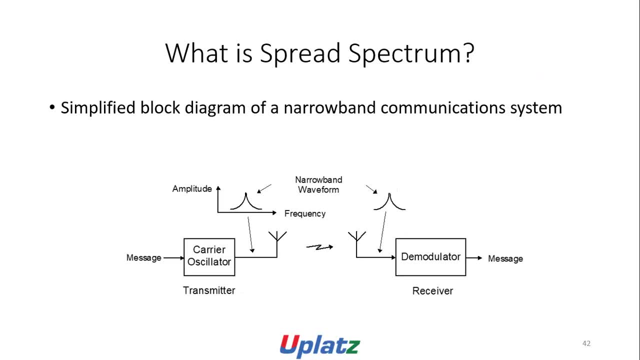 being transmitted independently from the information pairing. signal Reference interaction- spectrochromation by Peterson Zimmert and Boro Prenticeau in 1985.. Simplified block diagram of the spectrum waveform received by narrowband communication system: amplitude versus frequency shown narrowband. 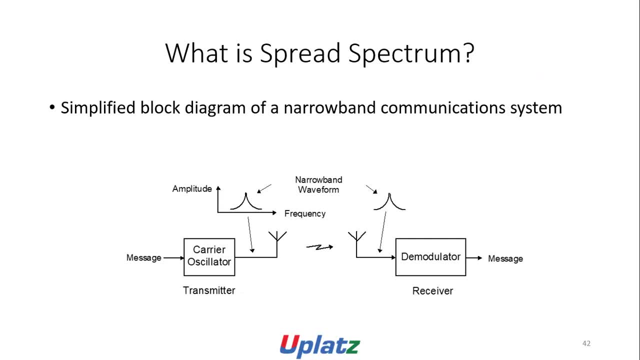 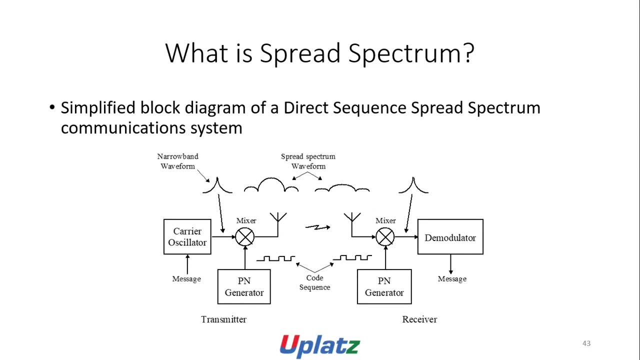 waveform message carrier, oscillation transmitter. then it goes to the remodulator where receiver and message is called back. Simplified block diagram: delta spectrum communication system carrier, oscillator, mixture p and zero random number generator. then transmit and spectrum waveform And receive the spectrum from the signal of the spectrochromic system to the 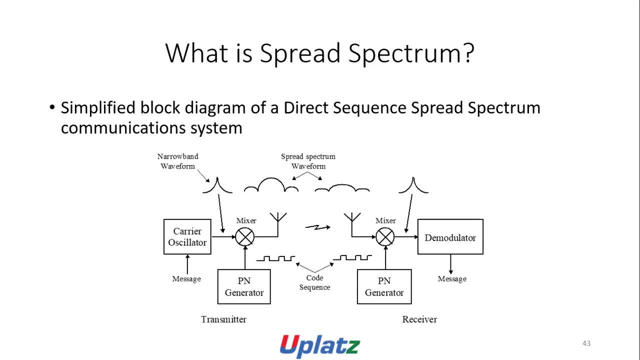 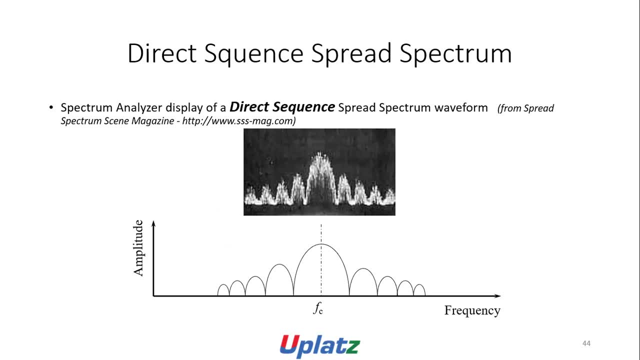 receive, mixture be generated, demodulated and the message is received. Spreadspectrum unveils a display of a direct-sequence spreadspectrum waveform for spread-spectrum scene magazine, As shown here. amplitude: there is a main lobe and there are side lobes of the same. 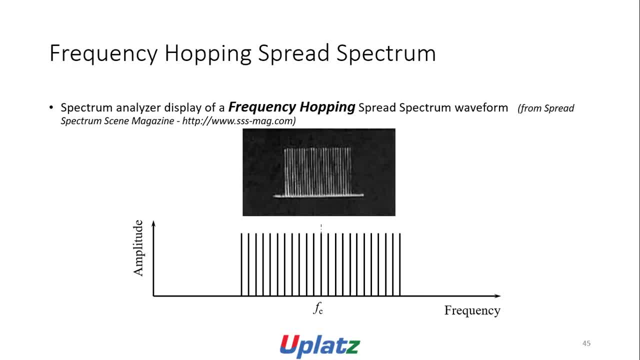 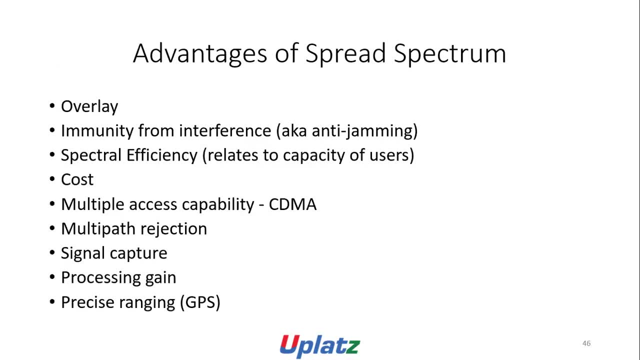 frequency. Frequency-hopping spread-spectrum Spreadspectrum unveils a display of a fluid-hopping spread-spectrum waveform as shown here. Overlay: immunity for interference at EKA: anti-jammies. pressure-spectral efficiency. reduced capacity of users. cost, multiple access capability- MA multipath rejection. 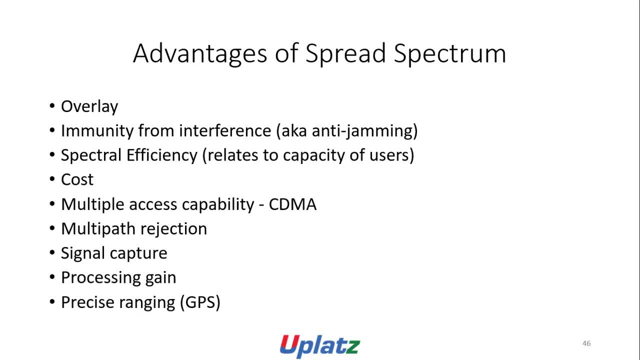 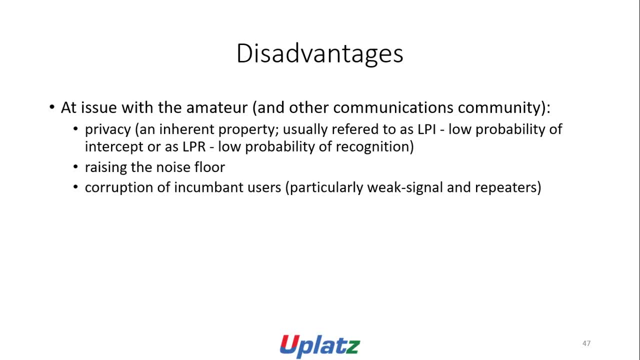 signal capture process range in GPS. This is an issue with amateur and other communication, community Private communication, Overlay, immunity for interference at EKA: anti-jammies, pressure-spectral efficiency, reduced capacity of users, cost, multiple access capability, MA multipath rejection. 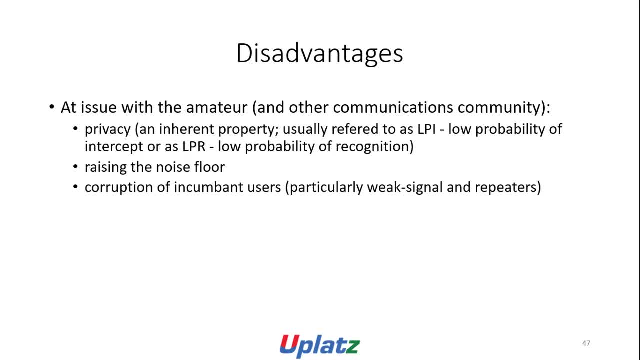 signal capture process range in GPS. This is an issue with amateur and other communication, community Private communication, Overlay, immunity for interference at EKA: anti-jammies, pressure-spectral efficiency, reduced capacity of users, cost. multiple access capability, MA multipath rejection signal. 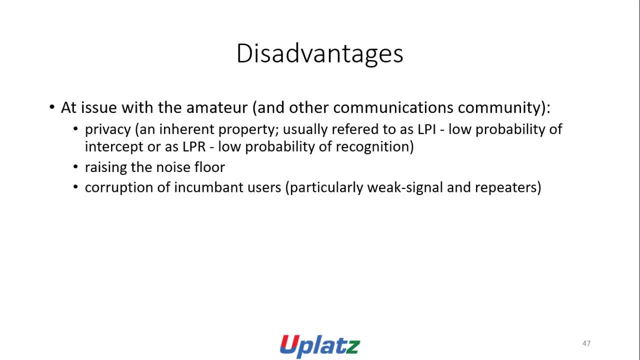 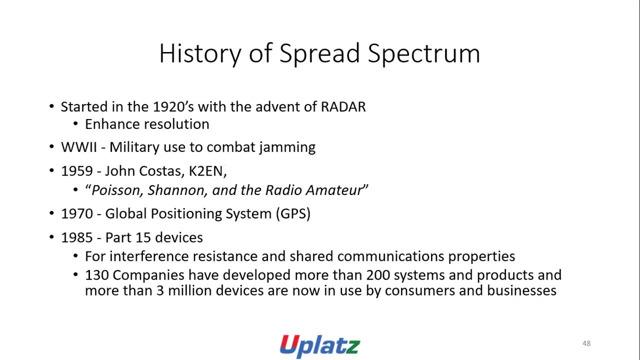 either non- 멋있able or non-visible, As seen here, although this is a fine contrast between the same controlled conversion. both have similar levels. Now what I want to do is to talk about the feedbacks that we have received on the 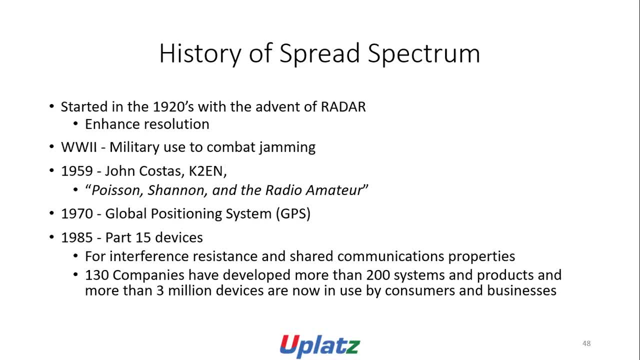 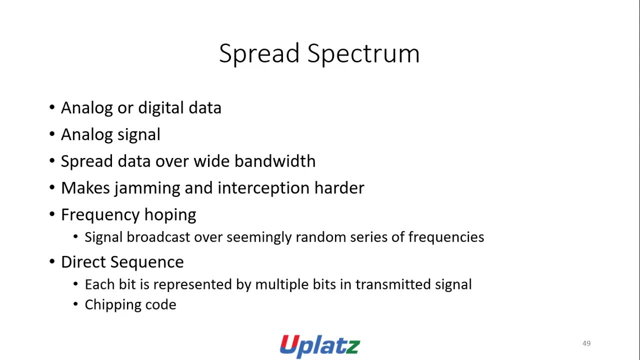 world map: question system 1985, part 15: devices for interference resistance and chat communication properties. 130 companies have developed more than 200 systems and products and more than 3 million devices are now in use by consumers and businesses. Spread spectrum, analog or digital data. 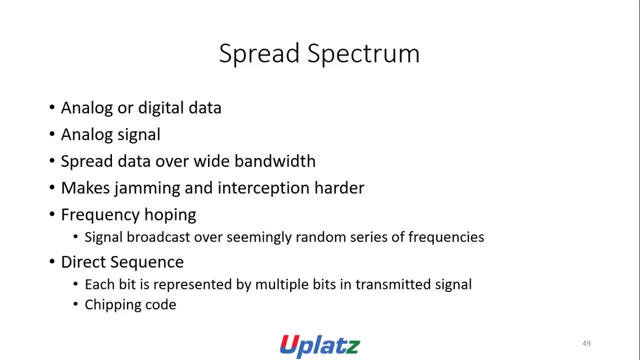 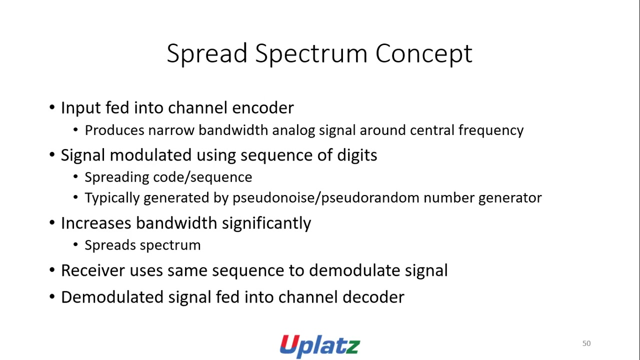 analog signals spread data over wide bandwidth, making jam and interception harder. Frequency, helping signal protocols more seemingly random. series of frequency: direct sequence: each bit is represented by multiple bits in transmitted signal. chipping mode: Input fed into channel encoder produces narrow bandwidth analog signal around central frequency signal. 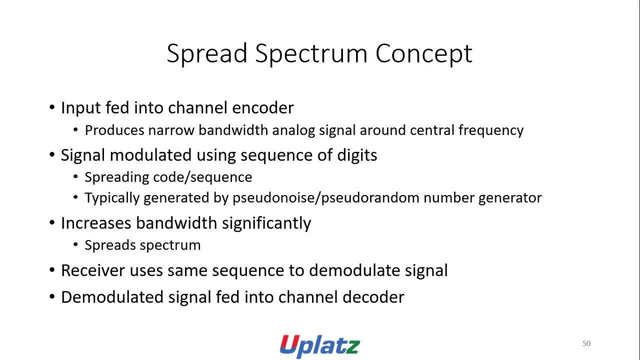 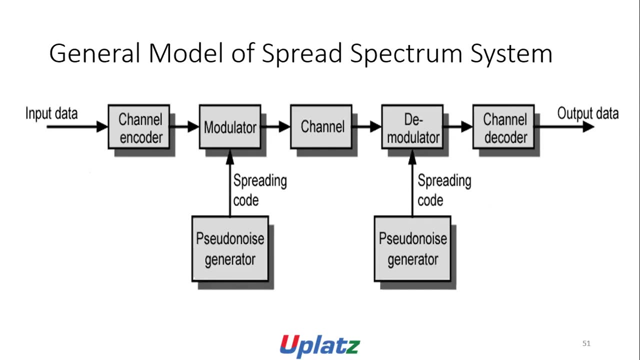 modulated using the sequence of gaseous spreading code: sequence difficult generator by pseudo noise. pseudo random number generator: increases bandwidth. segmental space spectrum received. use the same sequence to be modeled. signal fed into channel decoder: general model of a specific system. so input data: channel encoder modulator. 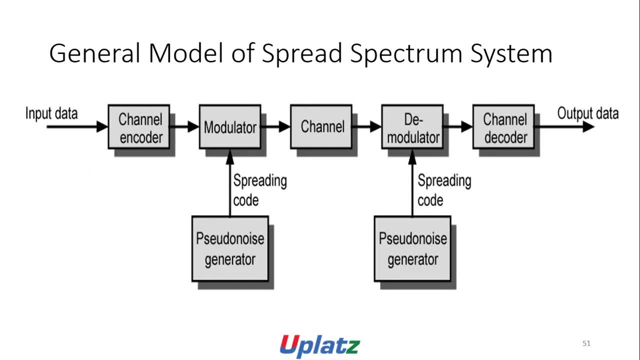 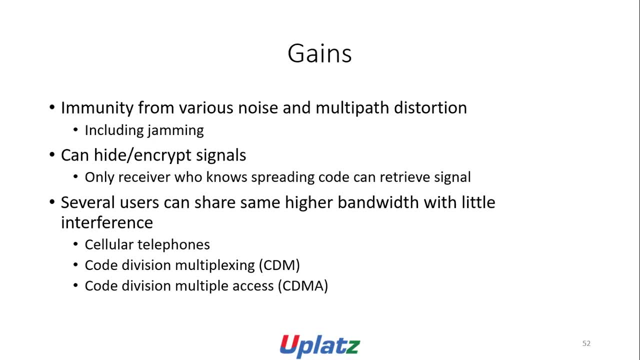 pseudo random data spreading code. channel demodulator. spreading code. pseudo noise generator, channel decoder and output data gains immunity from various noise and multiple distortion, including jamming. can hide input signals. only receive almost predict can. that is, several emotions can share the same high up and keep in playing. interference cellular. 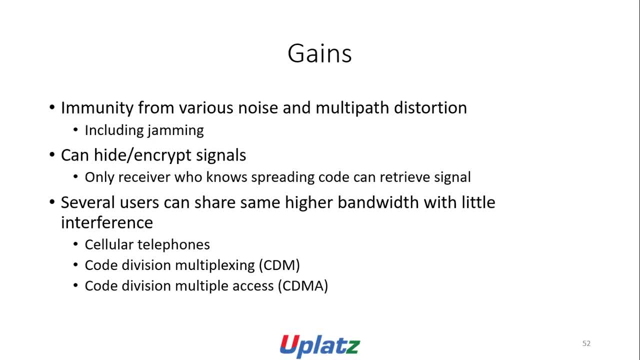 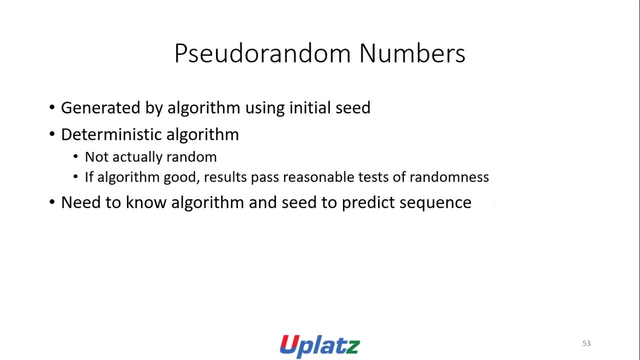 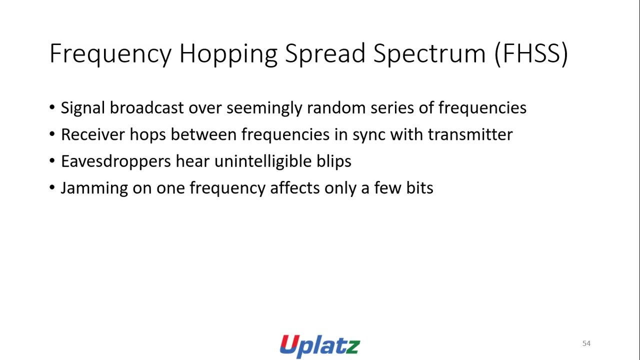 force code division. multiplexing code division, multiple access, pseudo random numbers generated by analog machine initial seed deterministic algorithm. not actually random algorithm code resource. also reasonable test of randomness. need to know algorithm and see it to predict sequence, frequency of being space spectrum signal, progress over seemingly random. 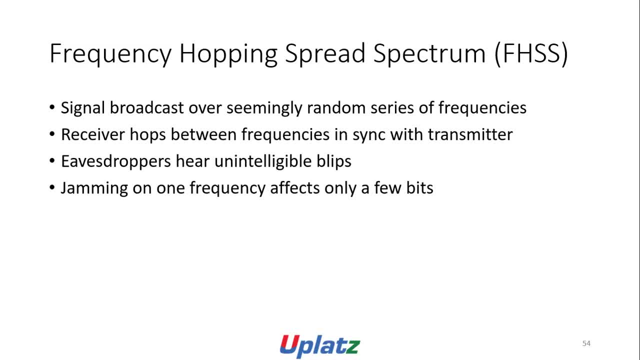 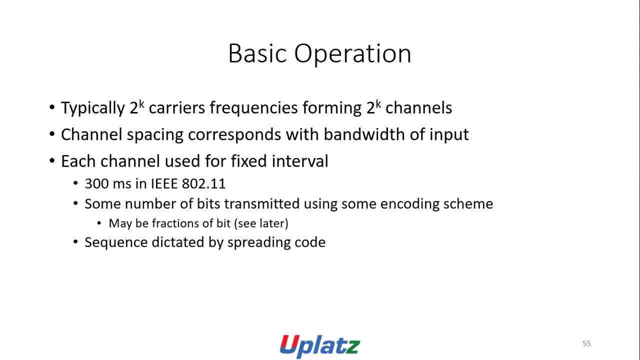 series of frequencies, receiver ops between countless800tors, with the eaves droppers here and until Glips Jamming on one frequency of X, only a few bits, basic operation, typically two cart carrier frequencies forming 24 channels, channel spacing, correspondence with bandwidth of input each and you'll spot x and interval to the millisecond in item be ignore. to point one one, some. 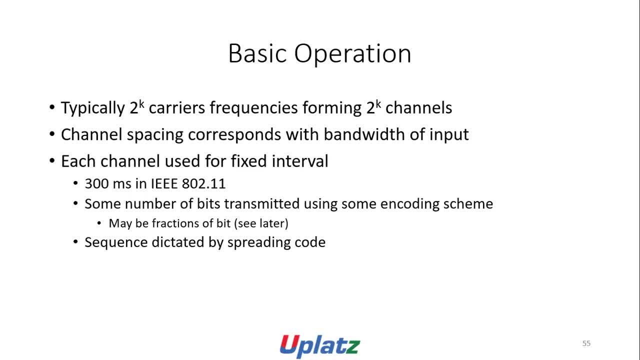 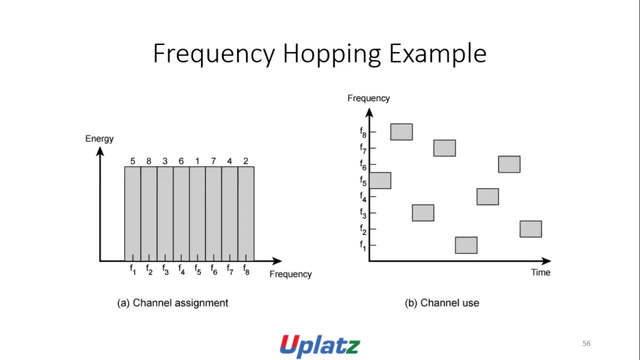 number of bits transmitted. you're using ultr isto faising skeptic Esc. some encoding scheme may be fraction of bits, sequence dictated by spreading code. The energy versus frequency for channel assignment and channel use are shown in figure. Channel use uses: time and frequency. Frequency of the spectrum system transmitter: binary data. 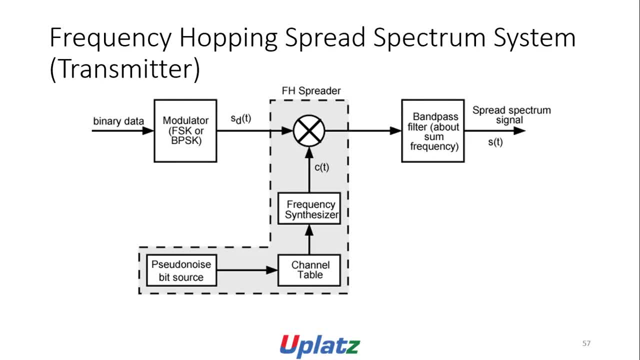 modulator FSK RBPSK. output of the modulator is spread to the pseudorandom bit source and channel table and frequency synthesizer CFT FS spreader, then bandpass filter about some frequency spectrum signal SFT is obtained. The receiver spectrum signal SFT is given and then pseudorandom 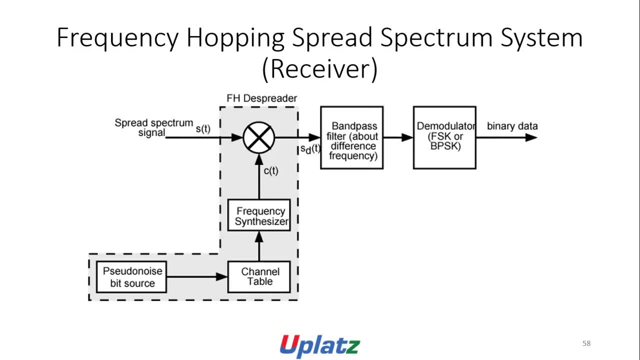 bit source, non-spec source channel table because they give CFT. they are mixed D spreader, STFT is formed, bandpass filter about difference frequency demodulator, FSK, RBPSK, and binary data is obtained. 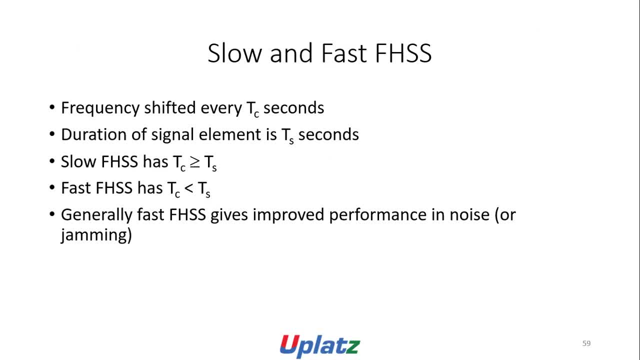 Slow and fast FHSS and FHSS Frequency shift in every TC-span duration of signal element is 10 seconds. Slow FHSS as TC-clad angle is 10 years. fast FHSS as TC: less than 10 years. generally fast FHSS gives more improved performance in noise or jamming. 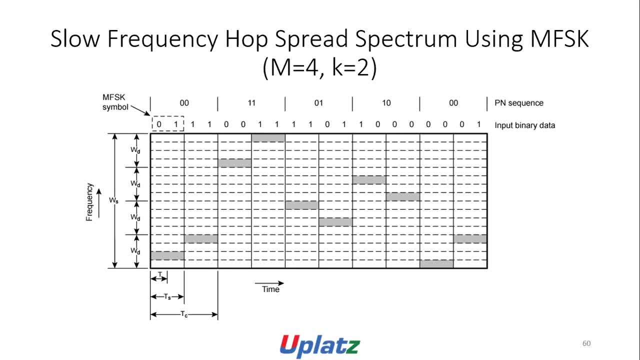 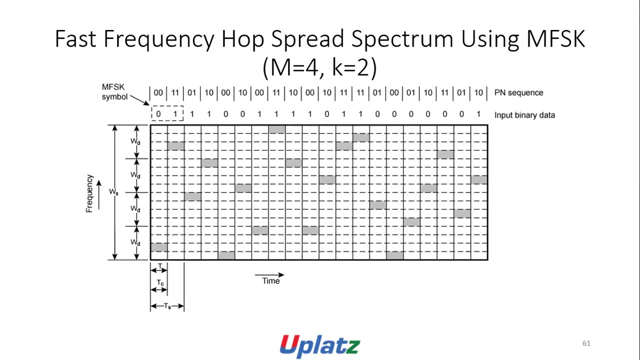 Slow frequency of spectrum using MFSK. M is equal to 4,. K is equal to 2, is shown in figure PN sequence and the binary data. y axis is the frequency and the u is the time For the different input sequences given in figure. what frequency of spectrum using MFSK. 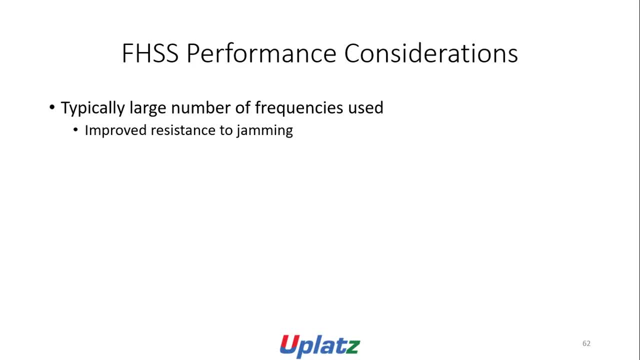 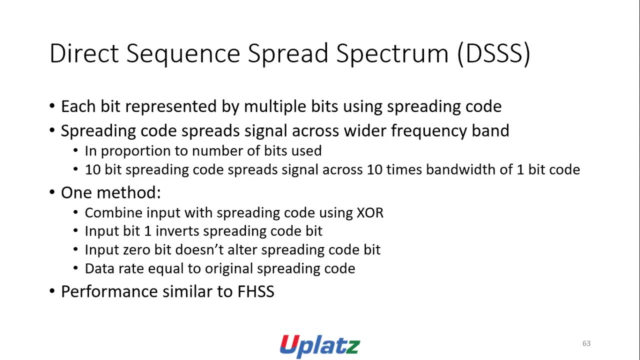 FHSS performance concentration. typically, a large number of frequencies use improved resistance to jamming. Direct sequence for spectrum. The time is converted to B-S- S-S. Each bit represented by multiple bits using spreading codes. Spreading code spreads signals across wider frequency band. 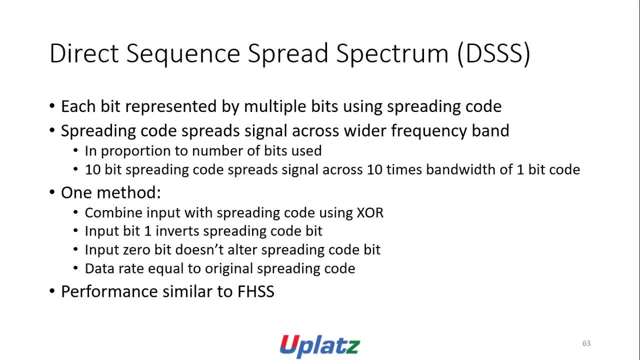 in proportion to number of bits used. 10 bits spreading code spreads signal across 10 times bandwidth to one bit code. One-by-3 combined input with spreading code. with UCXR Input, bit 1 inverts its spreading code bit. Input 0 will be descent. alter spreading code bit. 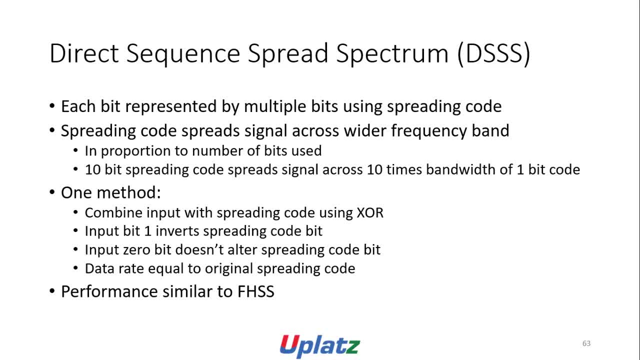 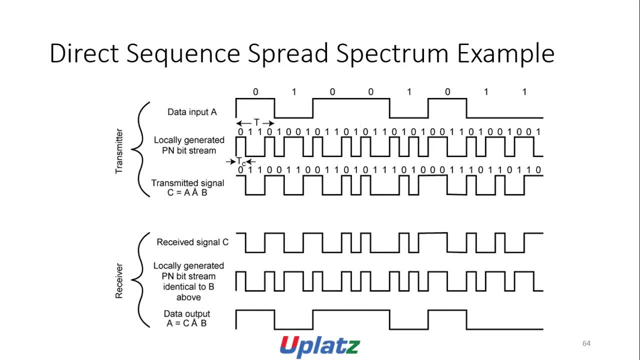 bit data rate equal to original spreading code. performance similar to FHSS Direct sequence specification. examples shown in the transmitter side and data input: locally generated PN bit stream and transmitter signal are shown and receiver receive signal: locally generated PN bit stream- identical and the data output are shown. 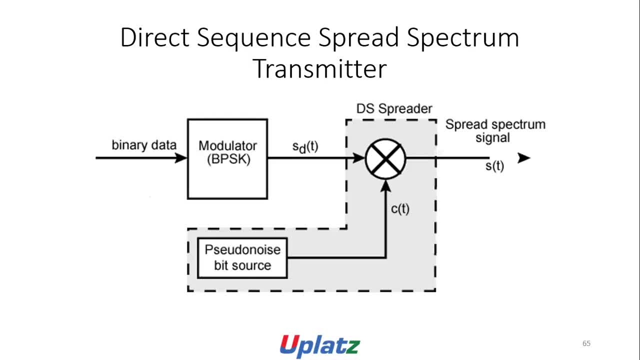 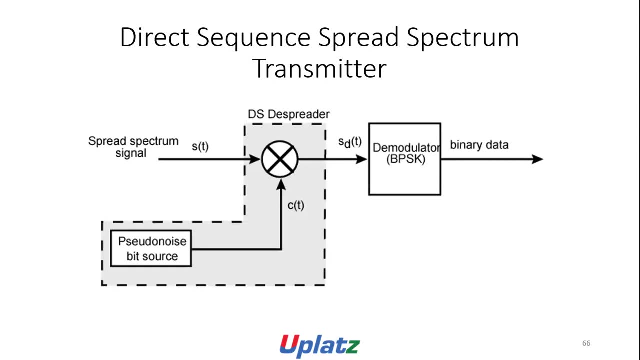 Data sequence specification. transmitter: binary data. modulator PPSK- pseudo random bit shows. they are mixed, the spreader is dead, spectrum signal is obtained, Spread spectrum signal is given and then de-spreader is used with pseudo random noise bit shows and then demodulator PPSK used to get the binary data. 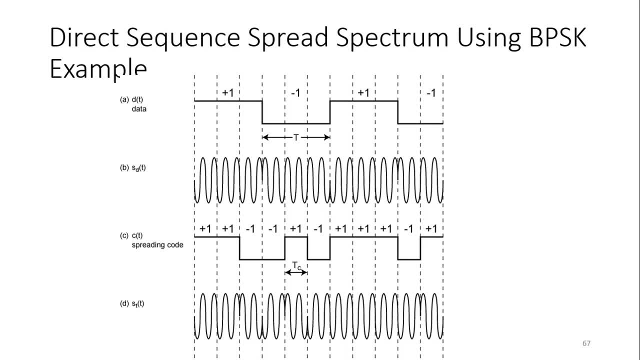 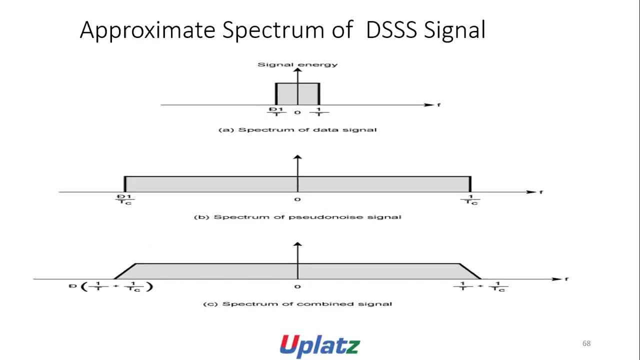 And data sequence specification. PPSK example: DT data. the SDT, CT and FTA waveforms are shown here. Approximate spectrum of DSS signal, signal energy is shown and spectrum of pseudo random signal and spectrum of combined signal. 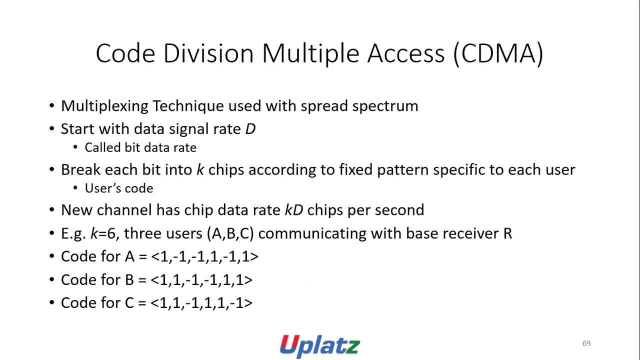 all are shown in this picture. One-division multiplexer: multiple access multiplexing technique used in the spectrum. start with data signal rate D, called bit data rate. break each bit into k chips according to fixed pattern specific to each user. 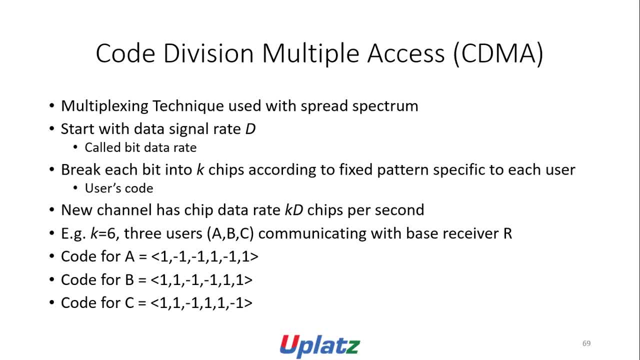 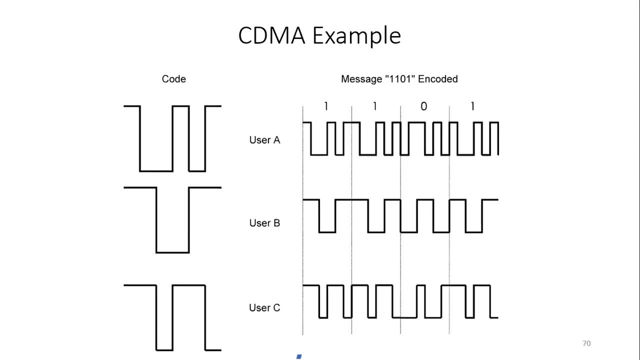 user's code: neutral analysis. chip data rate, KD chips per second. Example case with three users: ABC communicating with base receiver. R code for K, B and C are shown here. Message is encoded by the different users with a different code. 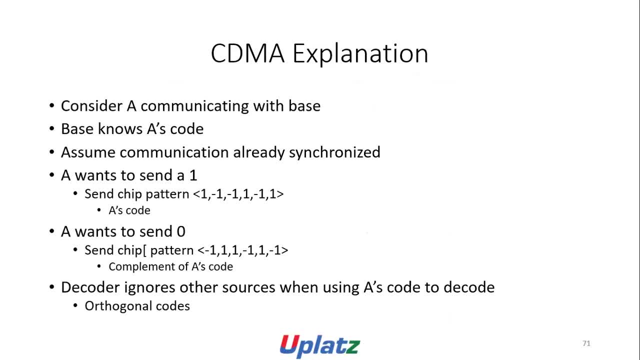 As shown in the figure CDMA explanation. considering A communicating with base base known AS code, assume communication is already synchronized. A wants to send A1, send chip pattern AS code. A wants to send 0, send chip pattern to get complement of AS code.